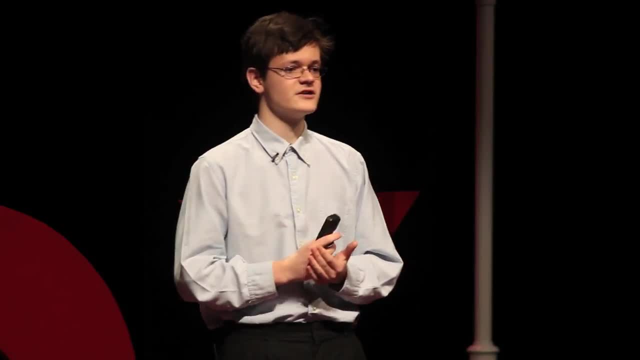 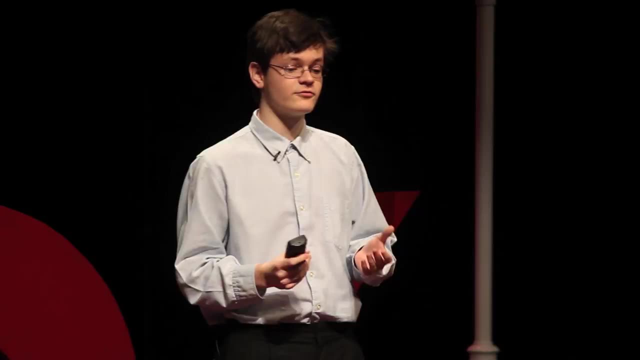 I want to touch on is if you want to learn something, you have to be interested yourself, You have to be motivated to learn, You have to be intrinsically motivated to learn, And there's no end of reasons why the Fibonacci sequence is interesting and why people would. 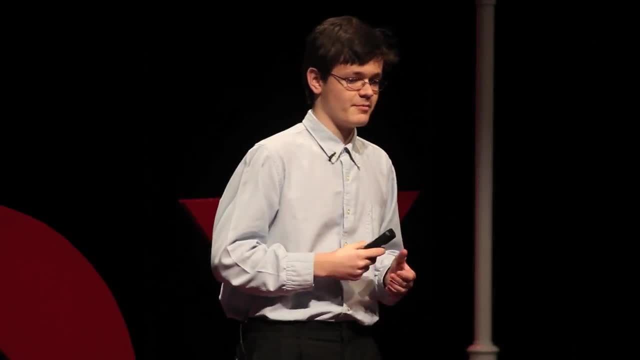 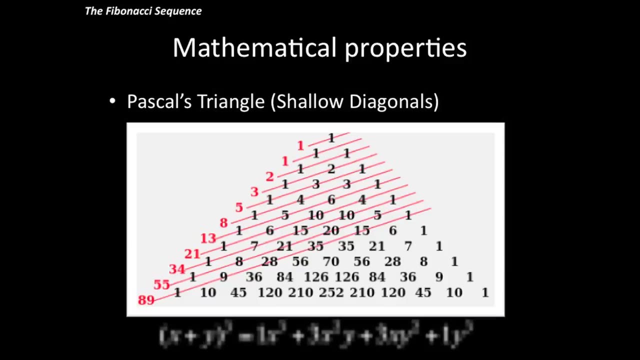 want to learn about it. There are a lot of mathematical properties for the Fibonacci sequence. Here's the first one I want to talk about. Pascal's triangle is used to expand binomials, So if you have x plus y cubed, you can see that the four numbers on the bottom 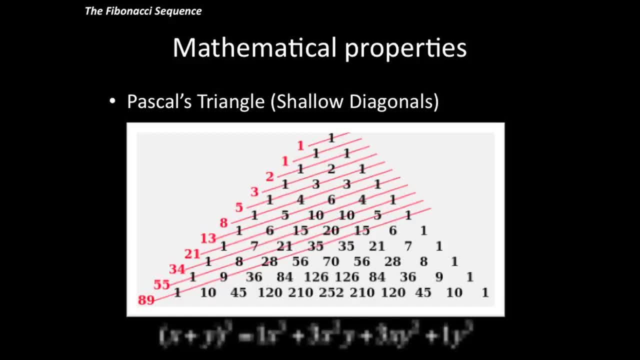 there 1, 3,, 3, 1,. those correspond to a certain row of Pascal's triangle, And that's what I'm going to talk about. But if you take the shallow diagonals of it, as you can see, 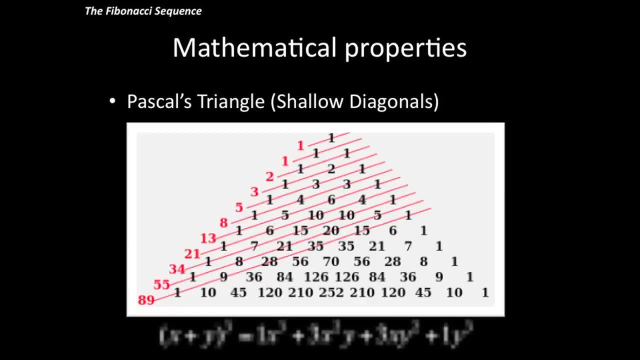 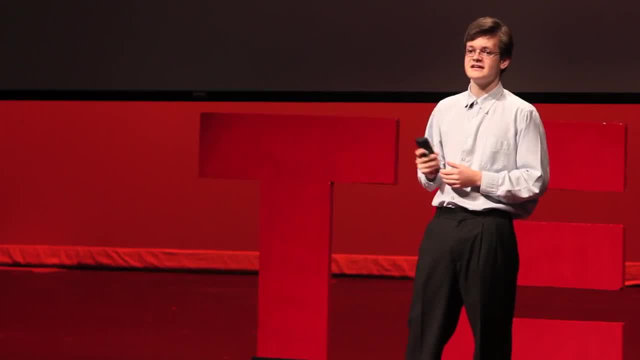 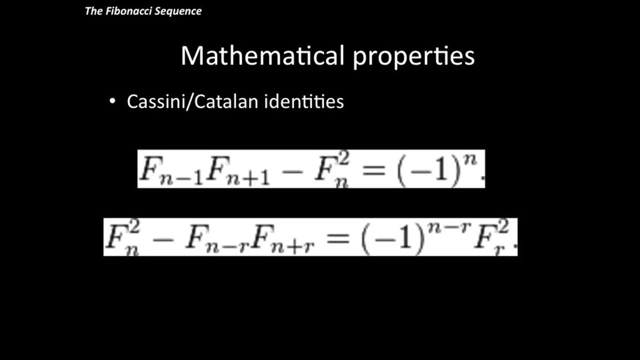 in the picture, those shallow diagonals. if you add up all the numbers, they will give you the numbers of the Fibonacci sequence. Another mathematical property: the Cassini and Catalan identities. The Cassini identity says that for any three consecutive terms in the Fibonacci sequence, say 3,, 5,, 8,, if you multiply the outer two and then you square. 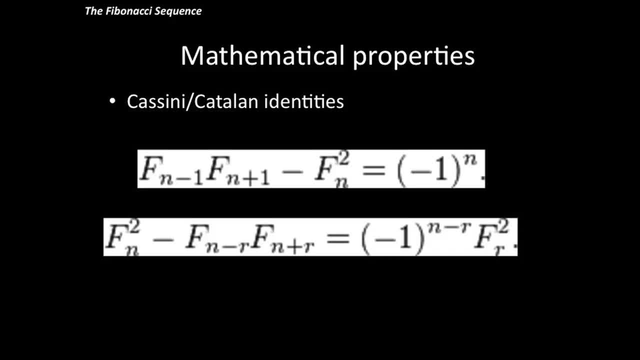 the inner one, they will differ by exactly one. So 3 times 8 is 24.. 5 squared is 24. 25.. They will differ by exactly one, no matter what three consecutive terms you pick. Zeckendorf's. 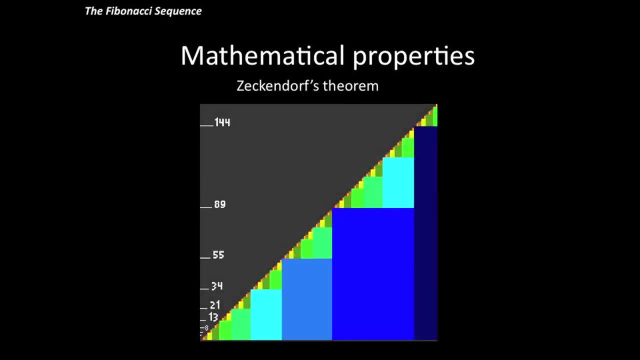 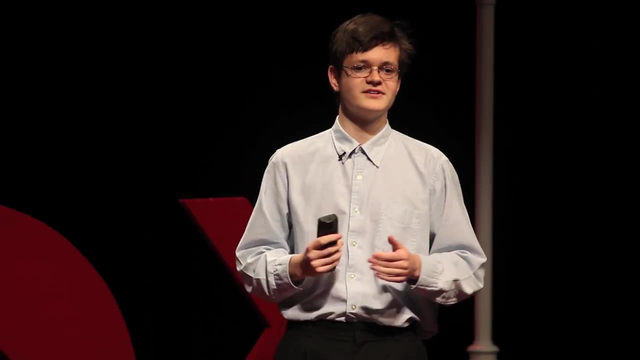 theorem says that any natural number you can think of, any natural number, can be arrived at by adding up different Fibonacci numbers without repeating any. So say you want to make 189 plus 8 plus 3,, 102,, 89 plus 8 plus 3 plus 2,, et cetera. Any number can be arrived. 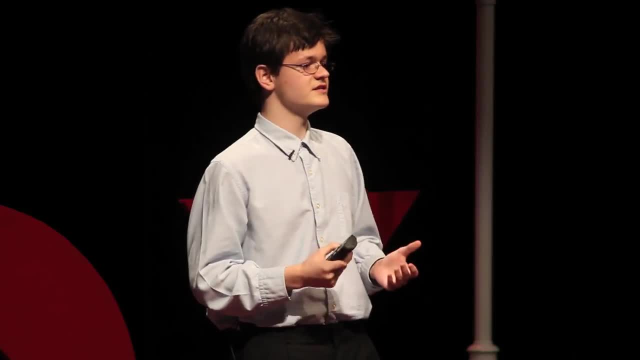 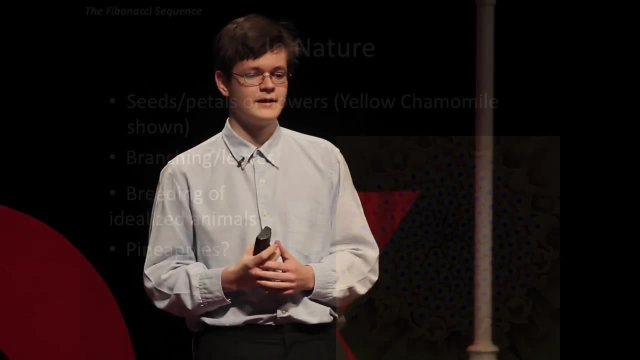 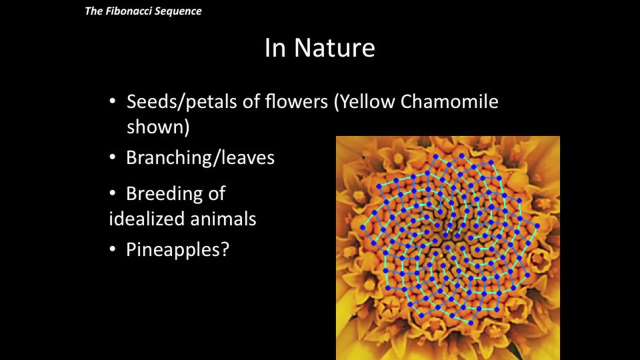 at in this way And in addition to these mathematical properties, which certainly interest me, a lot of people are interested in the Fibonacci sequence for their natural properties, The seeds in the petals of flowers. here you can see that they're arranged in a way that can be modeled by the 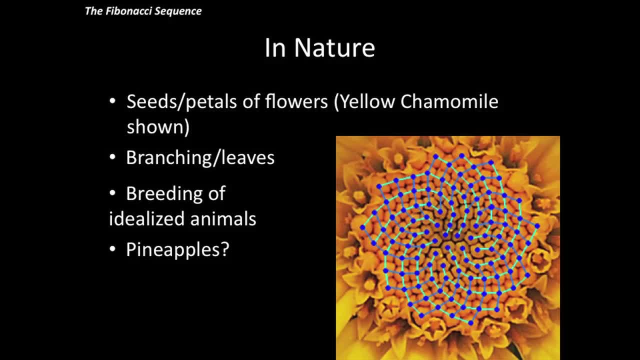 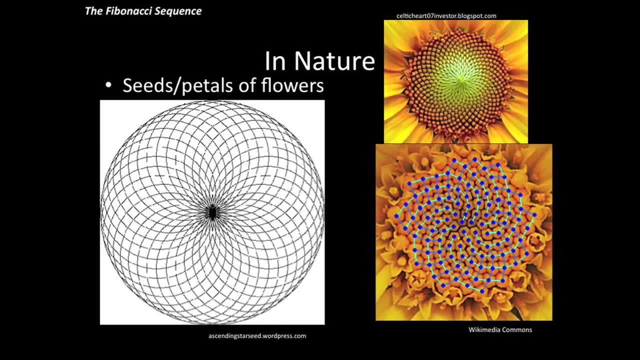 Fibonacci sequence and using a few of its properties. That's the model right there, in the bottom left, The branching of trees and leaves. if you have a tree, if you have a plant, oftentimes the number of branches at a certain level will correspond to the 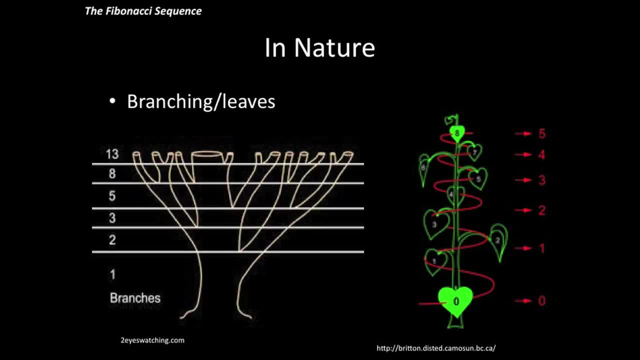 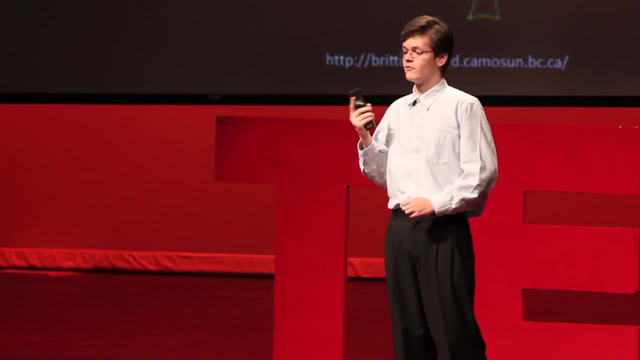 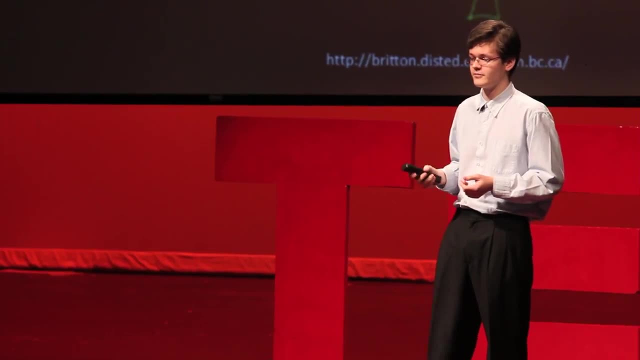 Fibonacci sequence, And if you have, say, a certain type of plant that has eight leaves on it that go around in a spiral, oftentimes that spiral will wrap around the plant itself five times And it's common for these to both be Fibonacci numbers. I skipped one, but there it is. This is actually how Fibonacci originally described the sequence with the breeding. 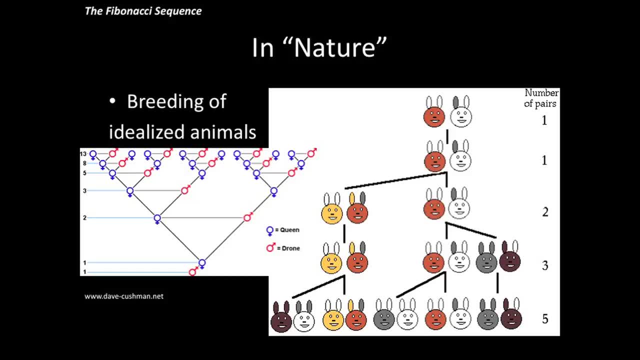 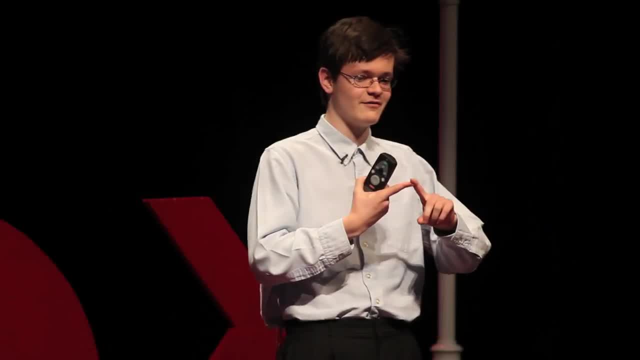 of these idealized rabbits. There's one pair of rabbits and then they mature and they produce another pair, who in turn mature and produce another pair. And these are, of course, very idealized. None of them can ever die. All of them produce exactly one pair every. turn, They all produce more rabbits at exactly the same time and you'd run in to all kinds of entertaining genetic diversity problems. But it's interesting. 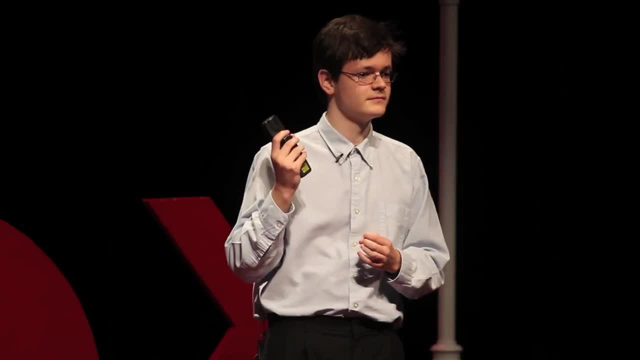 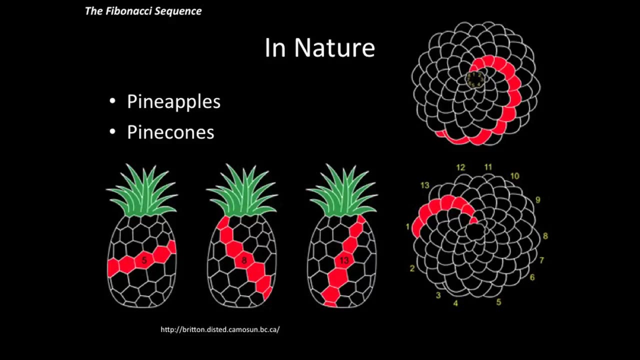 that this is the way it was originally described and that it works like this for a number of different animals. And finally, pineapples and pinecones, the spirals of them. You can see Fibonacci numbers in those, for example, in the different ways that you can. 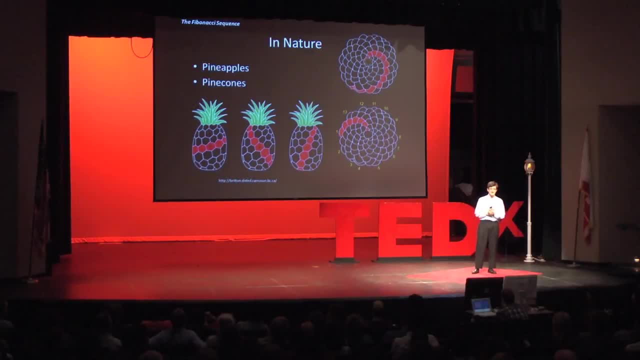 see a spiral in a pineapple or the number of spirals that you can see on a pinecone, But the main Fibonacci property that my talk is focusing on is this one: phi Phi is a number. it's 1.618 or thereabouts. it's an irrational number and it's 1 plus. 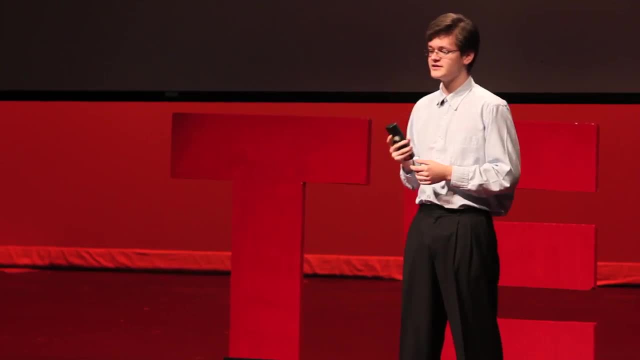 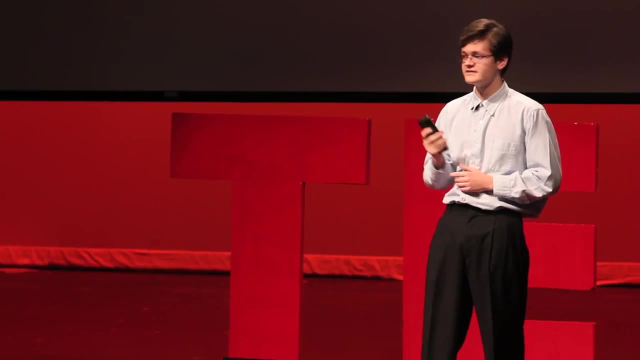 the square root of 5 over 2.. And the reason it's important is because it's the solution to both these equations: x squared equals x plus 1, and 1 over x equals x minus 1.. And it is also the converging ratio of the Fibonacci sequence. 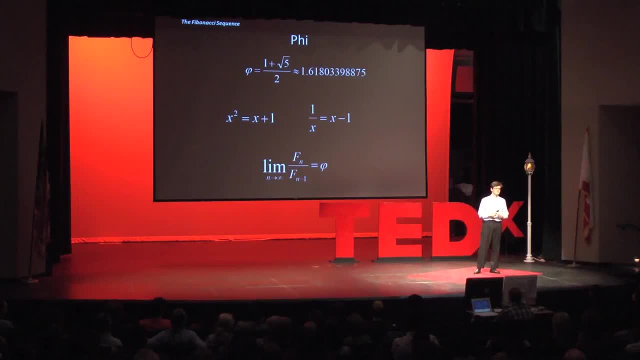 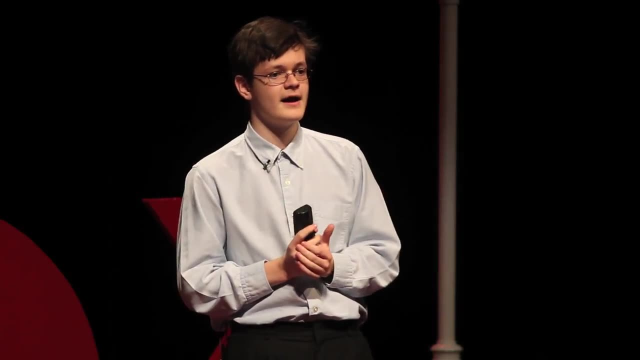 So if you go out to the infinitieth number of the Fibonacci sequence, it's a never-ending sequence. But if you take the infinitieth number and you divide it by the one before it, you will be left with phi. And that's what really interested me, is that this number, which is interesting in its own, 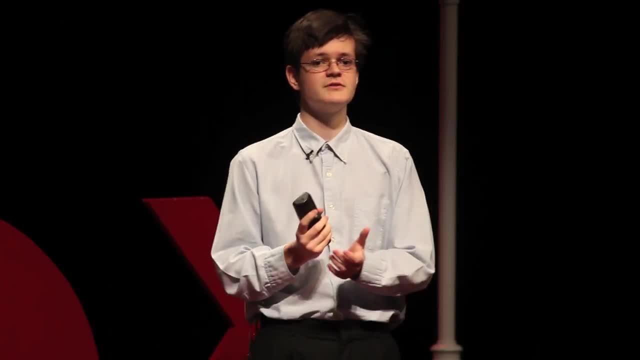 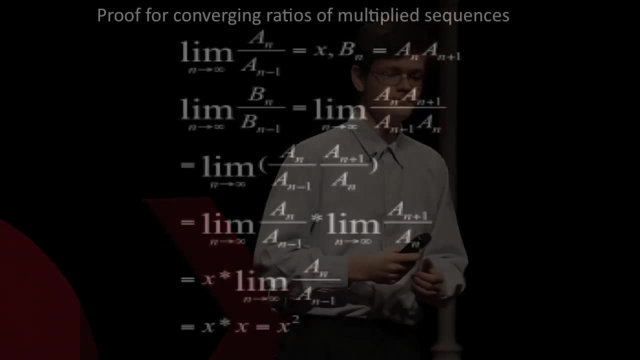 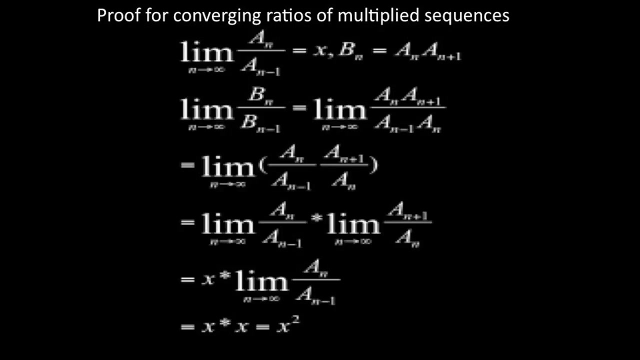 right, which is important in many branches of mathematics and which seems to be the human standard for aesthetics, is such an important number to such an important sequence. And here's where I want to talk about my experience, because what I did once was I wrote a program. 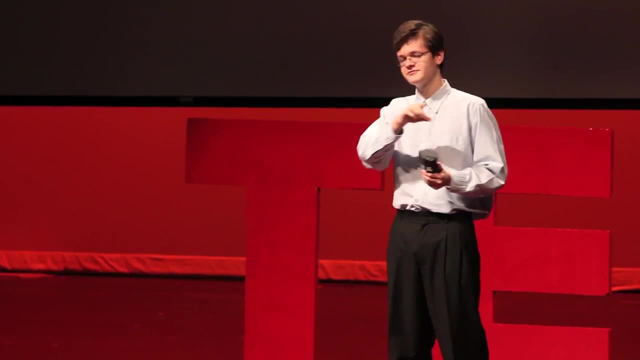 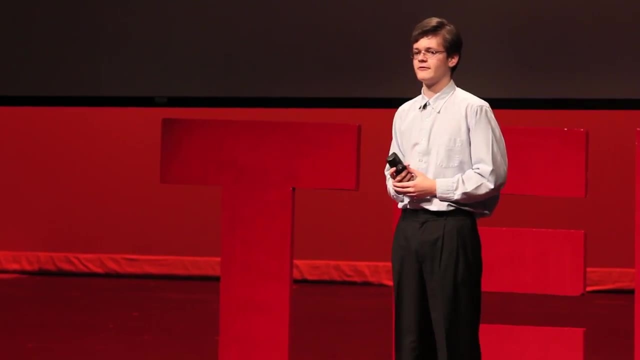 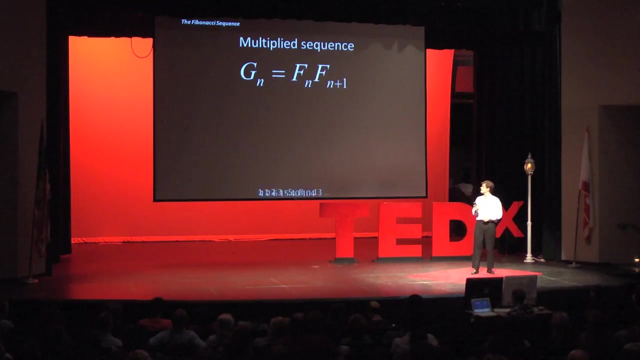 on my calculator to get phi. given the Fibonacci sequence, It's a very interesting graph that it traces about where the ratio gradually approaches phi. But then I turned it around And instead of dividing the numbers I multiplied them, And in that case you're left with a completely different sequence. 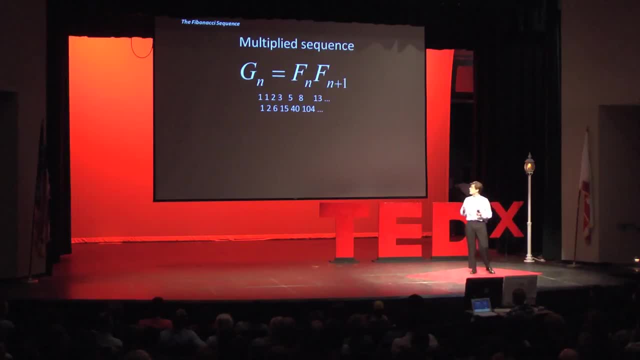 Since you're multiplying the consecutive terms- one times one is one, one times two is two, two times three is six, et cetera- And what really struck me about this was that the consecutive terms are not the same. They're not the same. 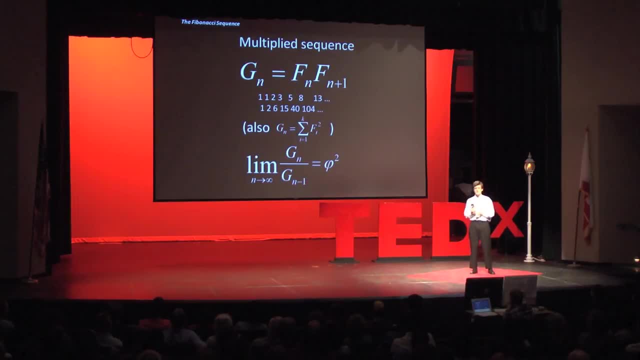 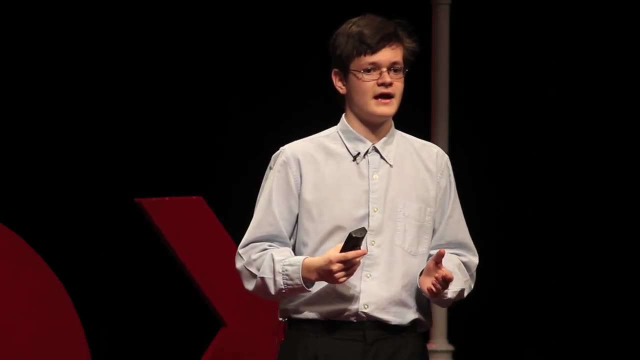 The converging ratio of that sequence is phi squared. And if you do it again, it's phi to the fourth, And then again it's phi to the eighth. And if, instead of multiplying two terms together, you multiply three, it's phi to the third. 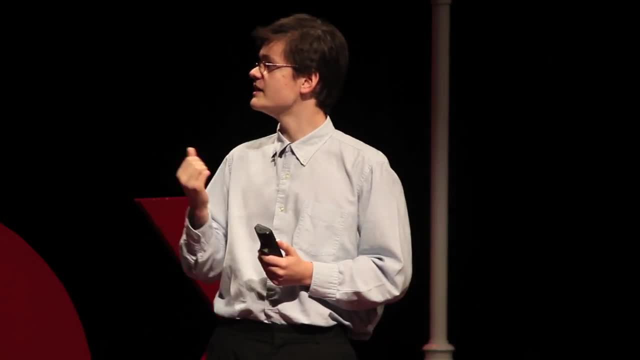 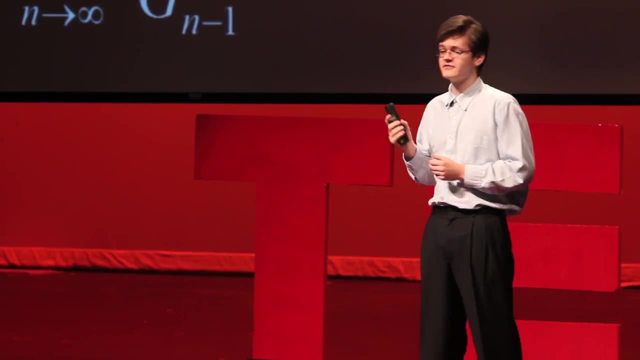 and then phi to the ninth. And that's what I thought was interesting, because in effect, this is like squaring the sequence: You're not actually squaring the sequence, but it's similar And the converging ratio is squared. Now it turns out that this in itself is not particular. 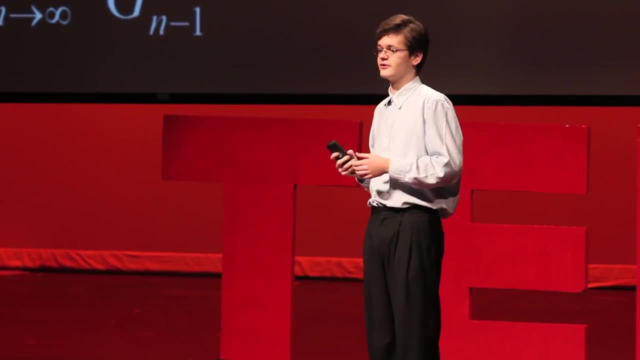 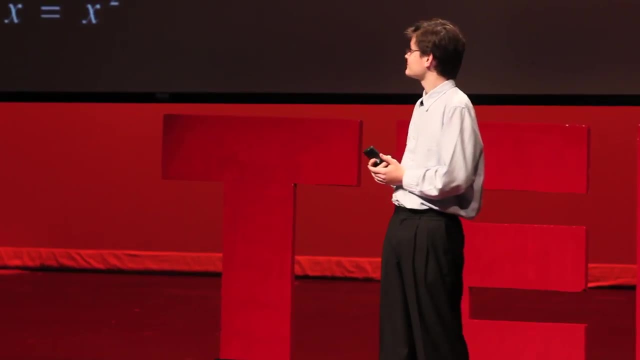 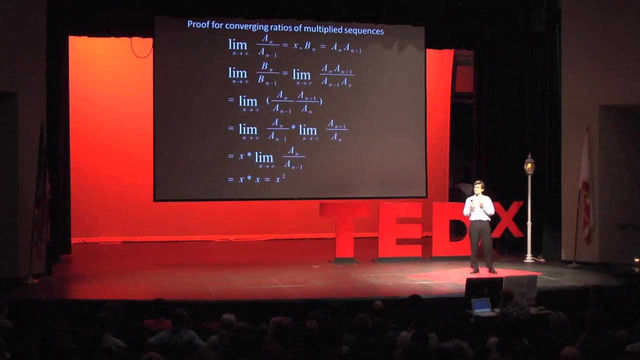 It's not the same, It's not particularly profound. The fact that this is true for any sequence with a converging ratio is short enough that you can fit it on a PowerPoint slide, And I did. But this is the first of three major learnings, three major discoveries that I had. 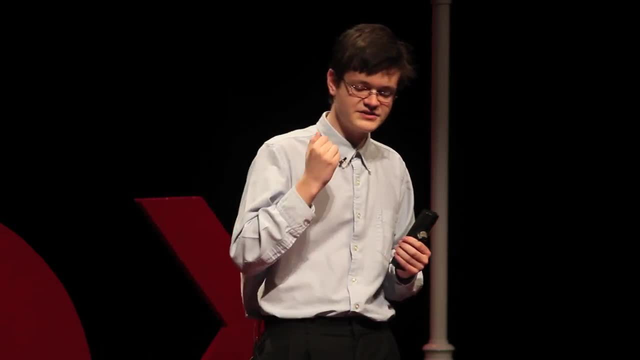 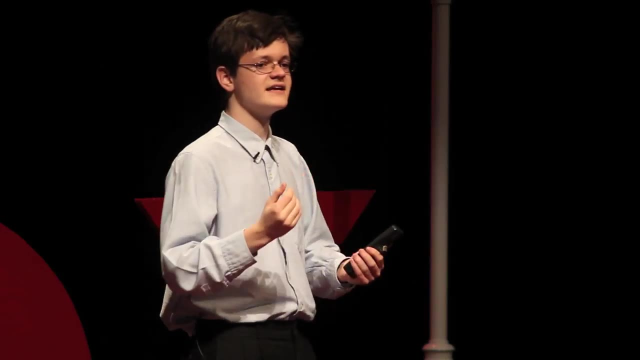 This is just the first of them, And what I want to say is: what if I hadn't come up with this on my own? What if we had been taught this in school? What if I had taken some class and they had either shown us this proof or even just given? 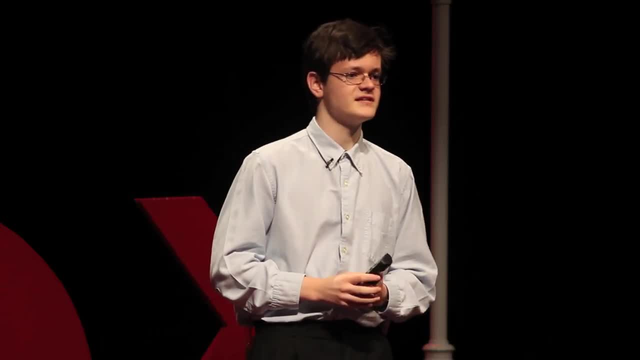 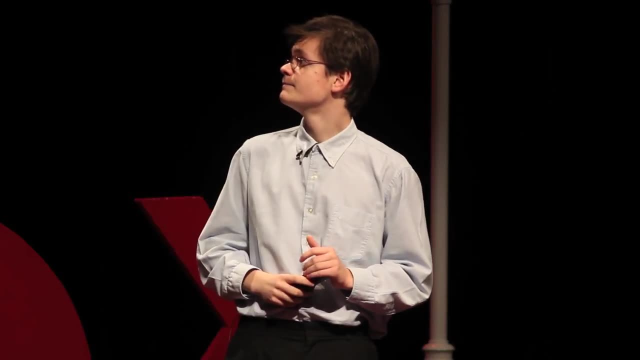 it to us, which is common, or even if we had gone through it step-by-step in class, Would I have continued? Would I have learned as much as I did? Would I have been interested in it? I don't think so. 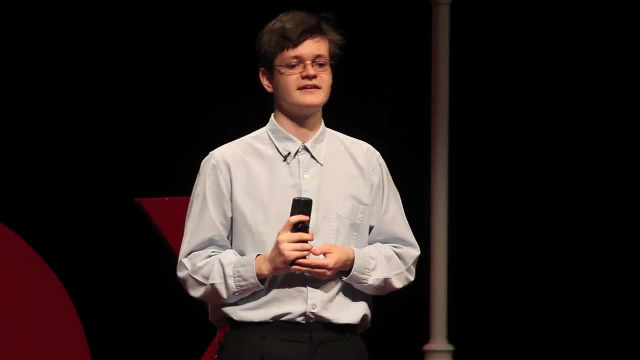 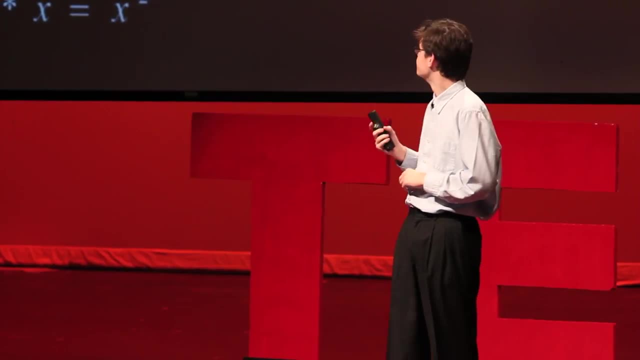 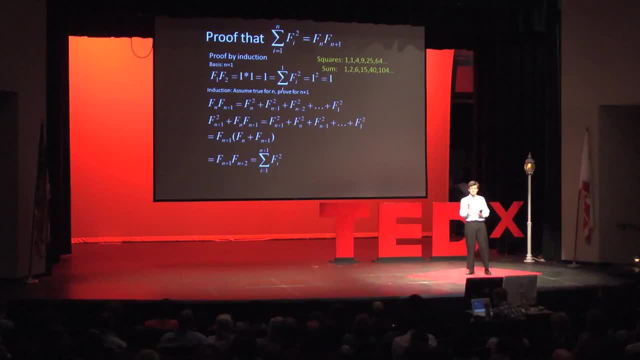 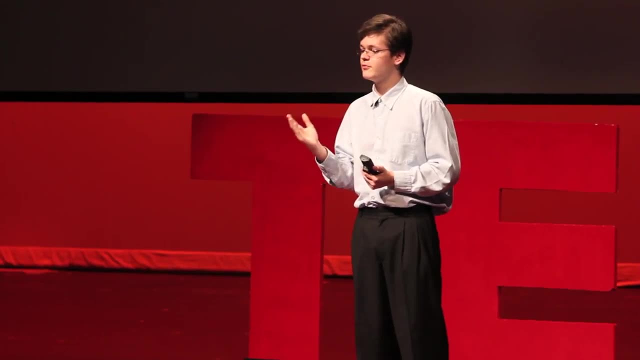 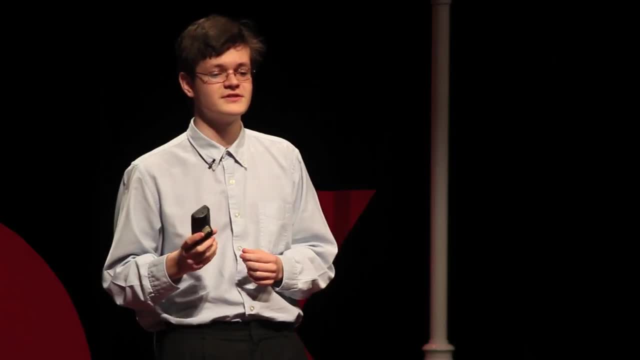 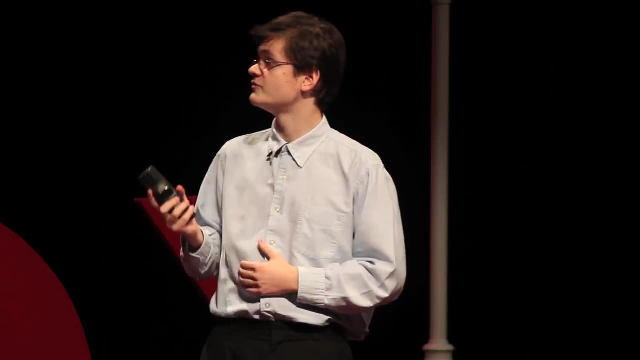 I want to think that was an EU cropped flag. And then that one happens between 10 keyconf and 11 keyed numbers And then it goes down and you measure it by how many keys you want. But that is a dangerous thing. It takes hours. 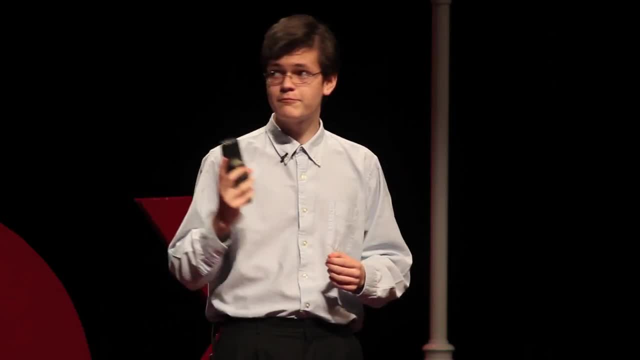 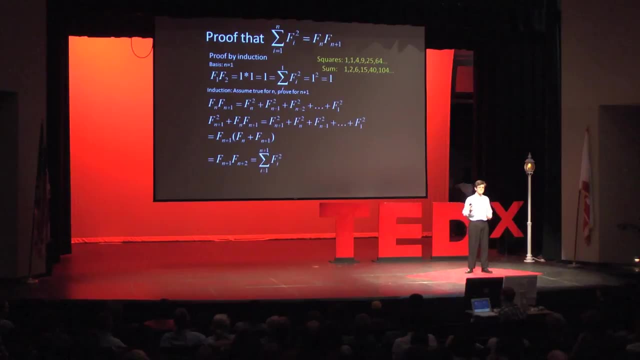 on mathematical sequences or on the Fibonacci sequence itself. I probably would have been taught this, But it's because I wasn't that I was able to really understand the thinking behind it and the way it works. It's because I was interested in it myself. 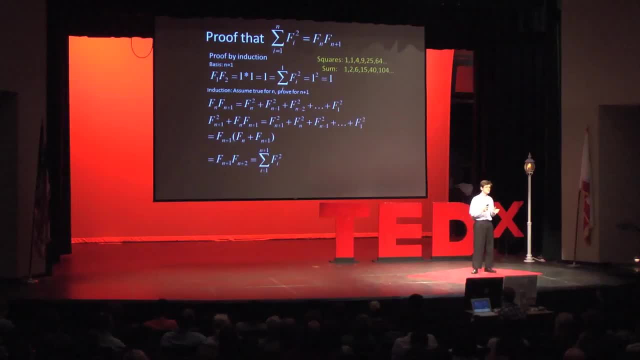 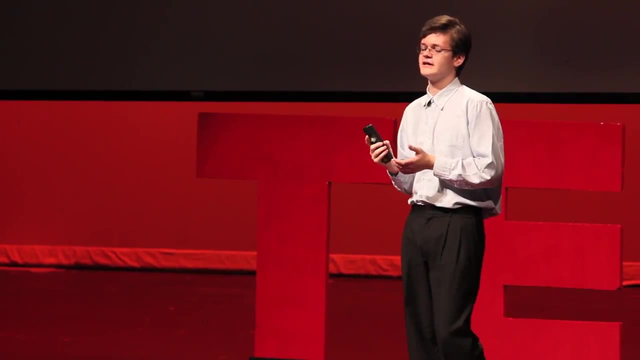 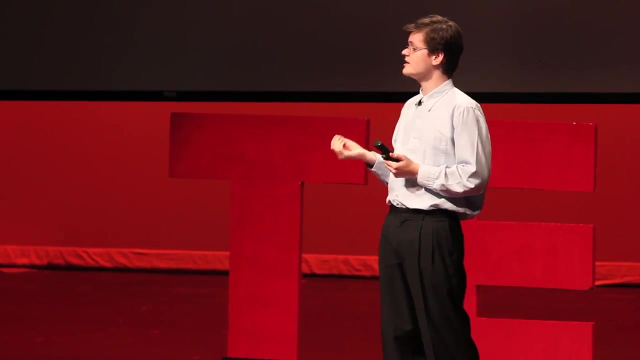 and I was intrinsically motivated. But the last one- and this is where I really found something interesting- is an explicit formula. An explicit formula is something that uses the number of the term, So for the Fibonacci sequence it's based on the two before it. 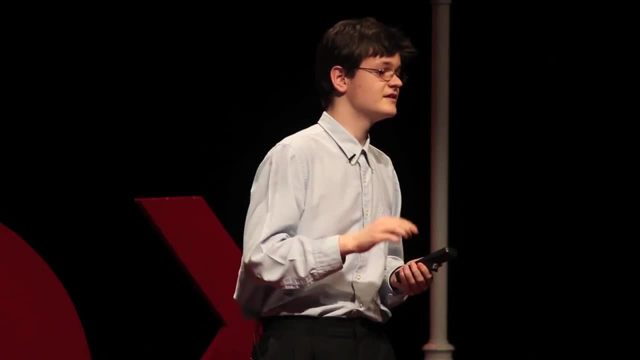 If you need to find the 100th term, you need to have the 99th and the 98th. If you need to find the 99th, you have to have the 98th and the 97th, And you can see where this is going. 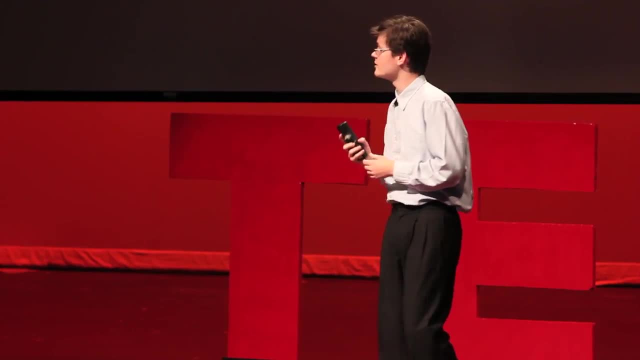 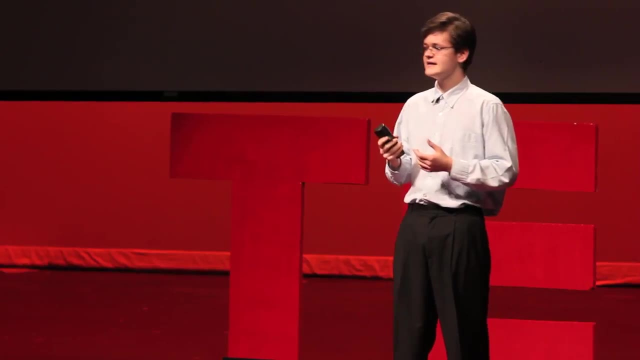 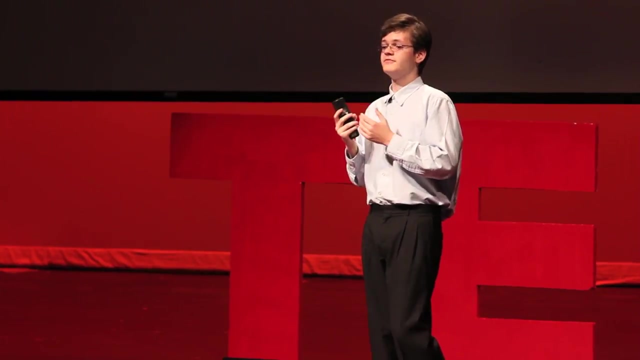 An explicit formula. all you need to know is that it is the term 100.. And there is an explicit formula for the Fibonacci sequence. It's called Binet's formula, And what I did is I set about using Binet's formula to have an explicit formula for any of these sequences. 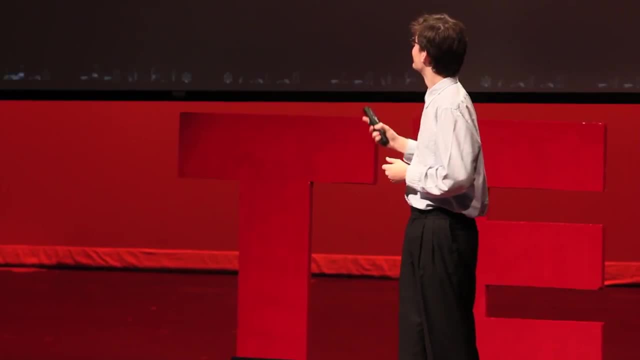 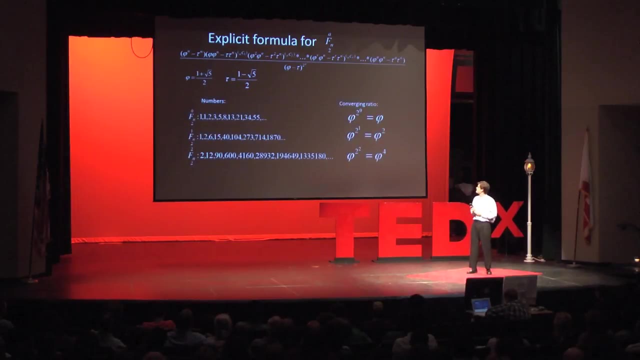 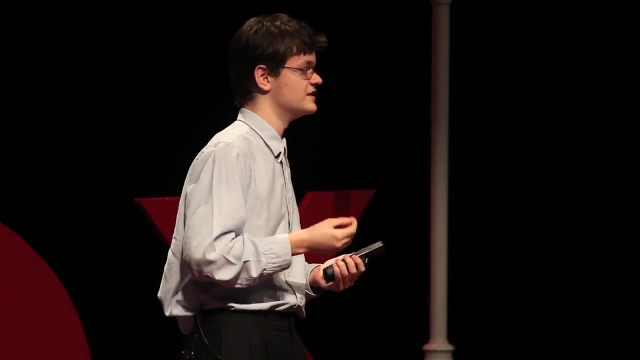 any sequence where it's been multiplied together. And there it is. It's rather long but it works, And it's for these sequences. A, which you see up at the top, there is the number of times that you've multiplied these terms together. 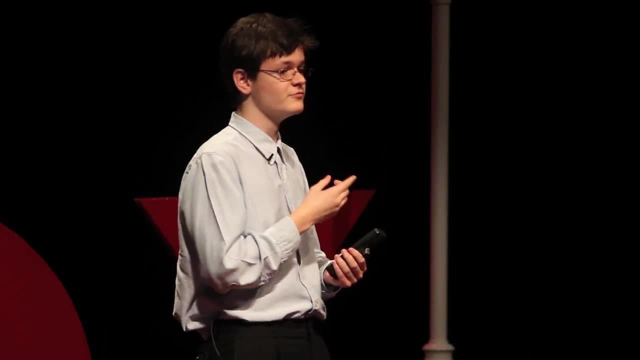 So if it's 0,, it's 0.. If it's 0, it's just the Fibonacci sequence. If it's 1, you've multiplied it once, If it's 2, twice, And you can see that the converging ratios follow that pattern. 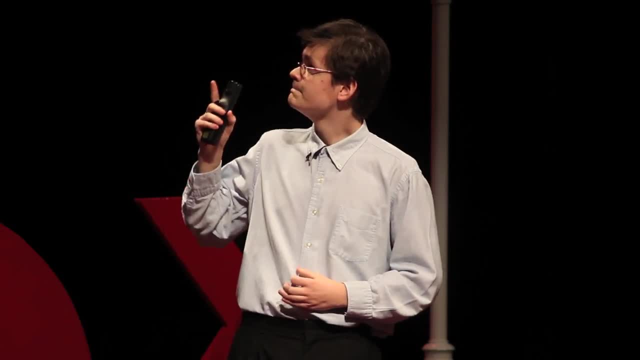 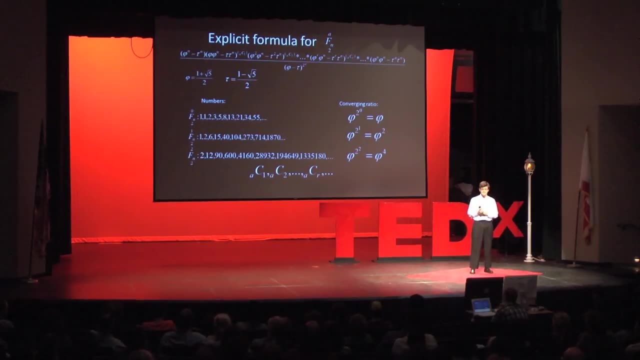 But the real interesting thing, the really interesting thing that I want to touch on, is if you look at the exponents of the numerator there, they follow this pattern: It's lowercase a, or rather it's a in a subscript, capital C1,.